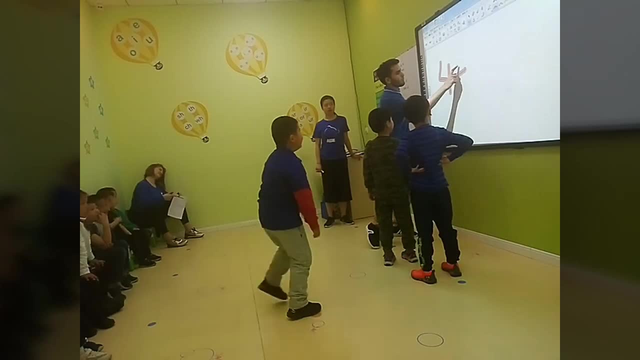 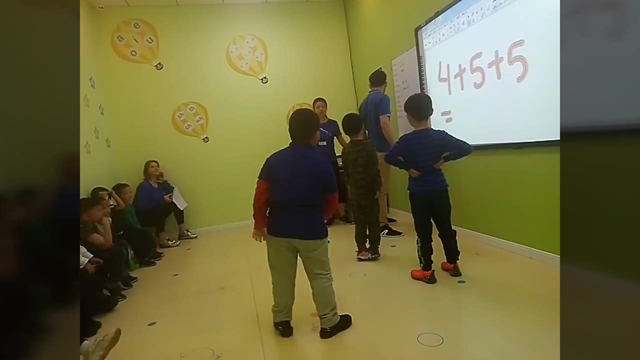 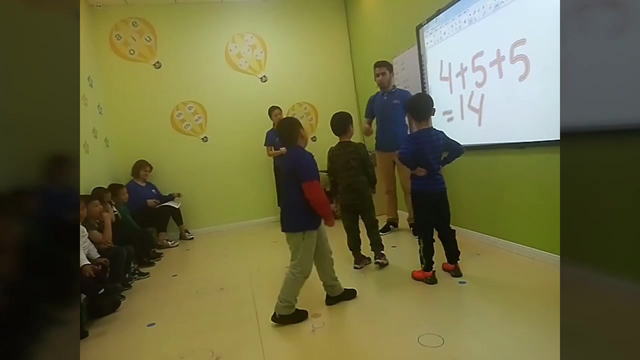 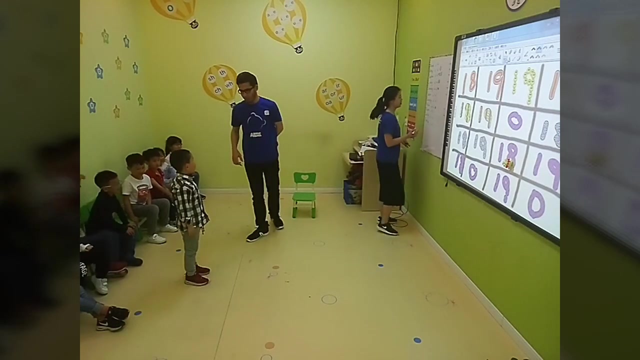 five. Wait, Four plus five plus five equals Fourteen, Equals fourteen. Very good Fourteen. You got it right. Give me five, Okay, Okay, Five plus five plus five equals crisis. One, two, three. Who are you already? 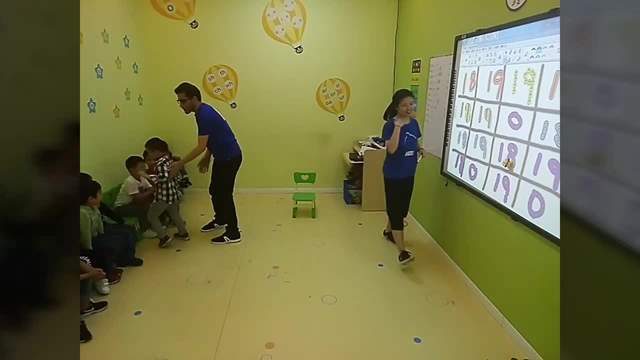 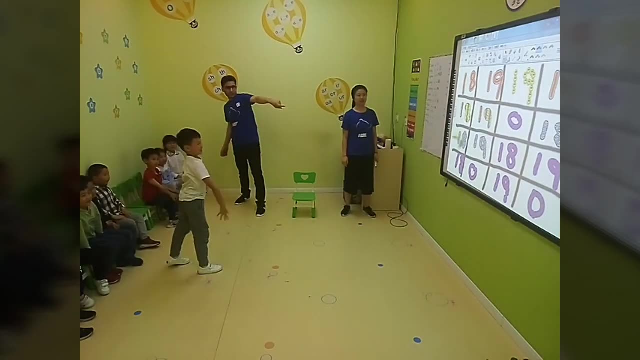 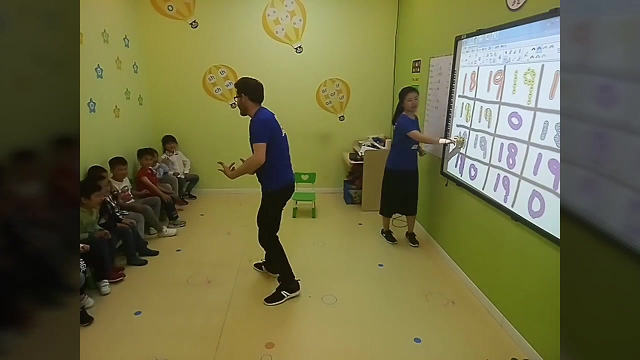 Here it is, Rock scissors paper. Oh, it is awesome. One, two, three, You got it right. loser items: Men, grab those little shadows of a man's mind and chase him. That's it All, right. 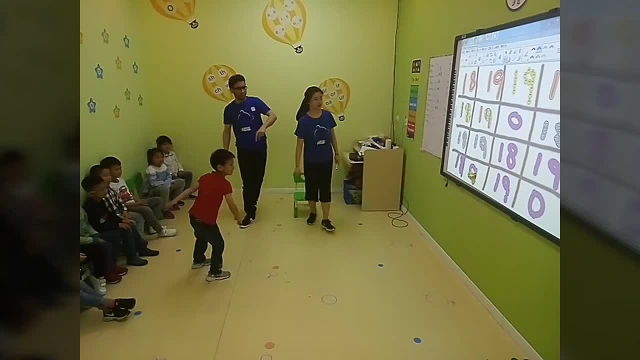 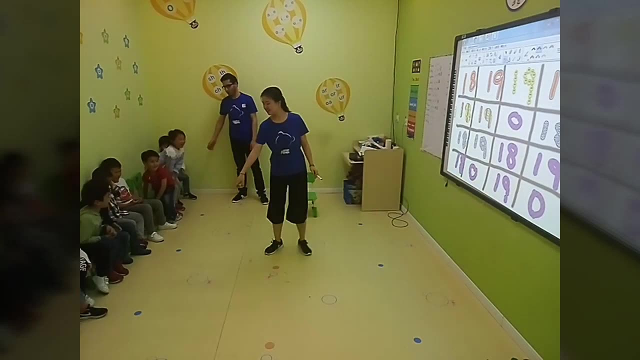 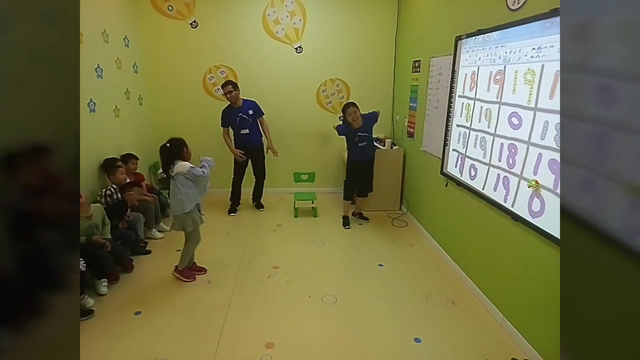 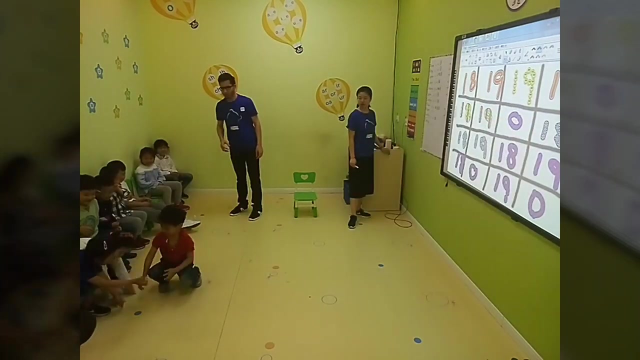 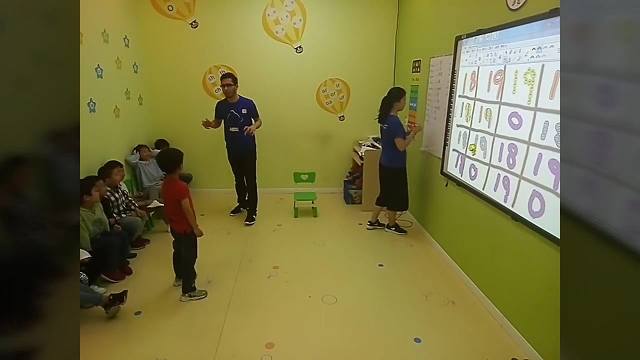 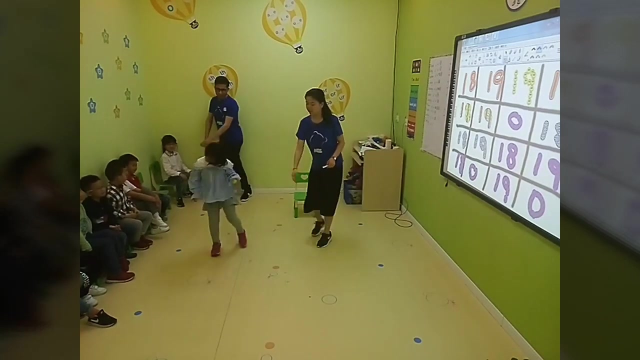 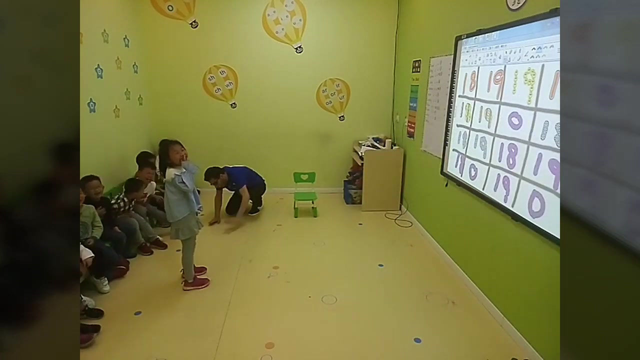 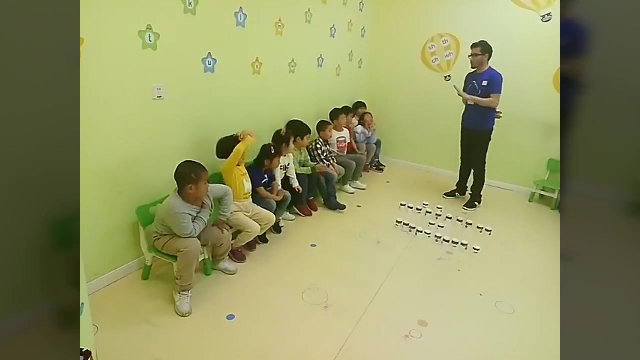 One, two throw hit. What number is it? Ready go, What number is it? Is it number 19?? What is his turn? Ready go Game. number 3 with cups. Number 18, number 19: I have cups numbers from 1 to 10 and from 1 to 10 there. 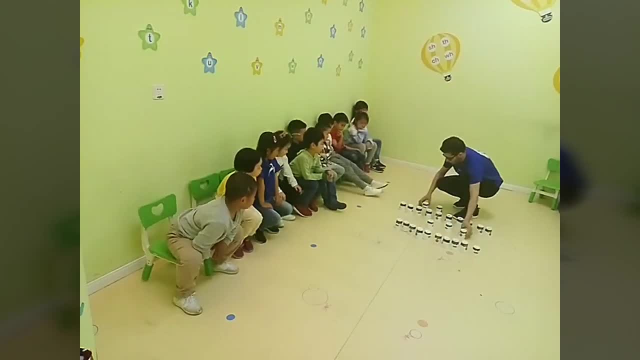 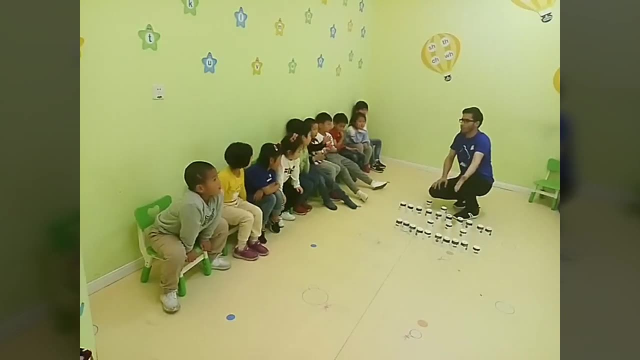 We have plus Plus here And we also have equals 18 or 19. I'm going to write numbers here on the board. You have to find the same numbers put in order and say it: 6 plus 4 plus 8 equals 18, like that. 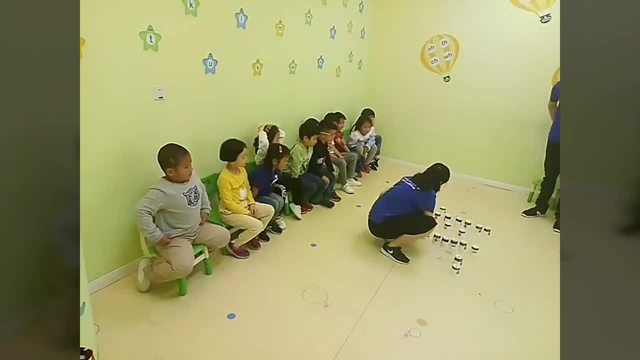 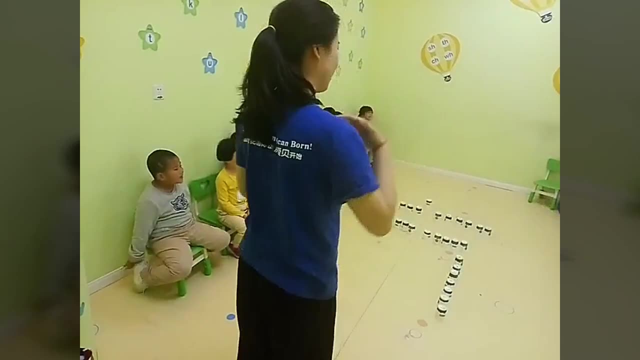 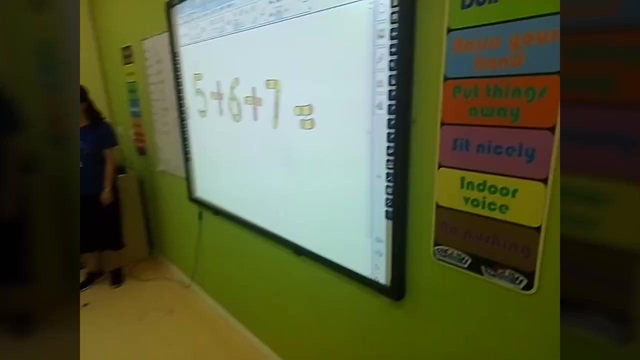 10 plus 6 plus 4 plus 9 equals 19, So I'm going to write 19 here, Guys. guys, look, 6 plus 4 plus 9 equals 19. You guys, let's try it. Magic: 5 plus 7.